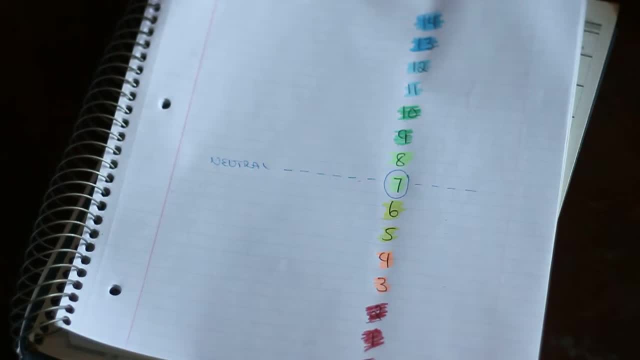 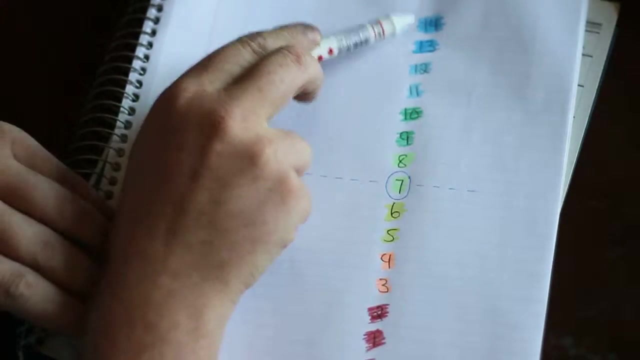 Hi everyone, and welcome to another episode of Garden Basics. Today I wanted to talk to you about pH balance. It's really important when you're gardening to know what your plants need in terms of pH. Essentially, what it is is the measure of the acidity, or alkalinity, in your soil. Now the scale runs from 0 down here up to 14.. So 0 is going to be your acids, 7 will be your neutral, and going up through 14 is going to be your acidity. 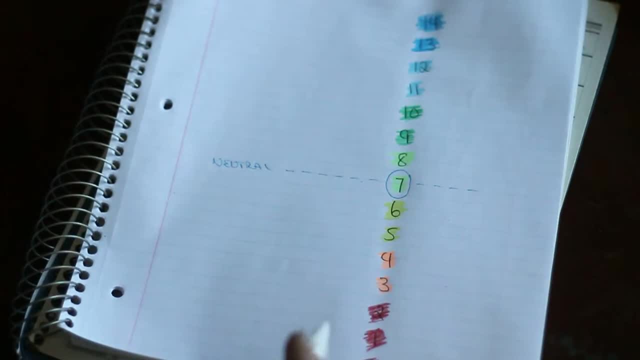 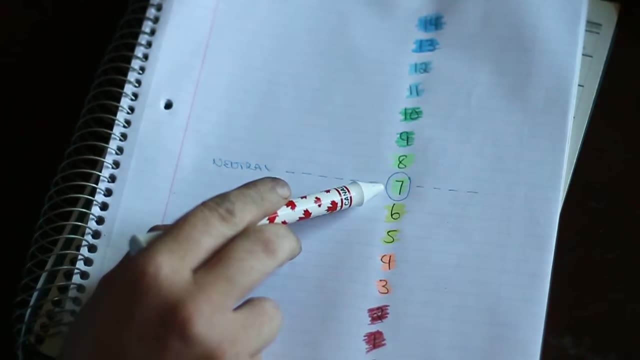 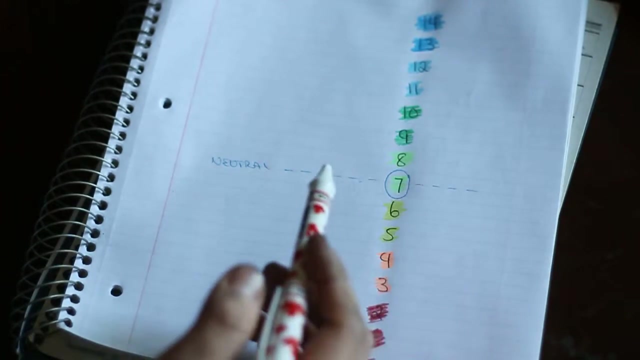 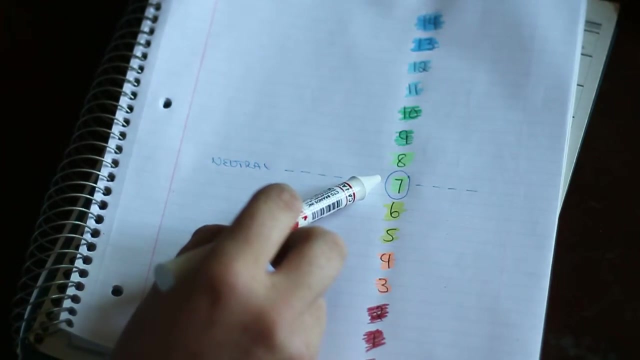 Now most people are going to be somewhere in between the 6 to 7 range, just their natural garden soils acidity level. So that's a little bit more on the acidic side, which is fine for virtually everything. But there are ways to amend your soil, either going down or up, depending on what you want to plant. Now, if you wanted to raise your pH level, there's a few things you can use. You can go with what is known as pH balance. 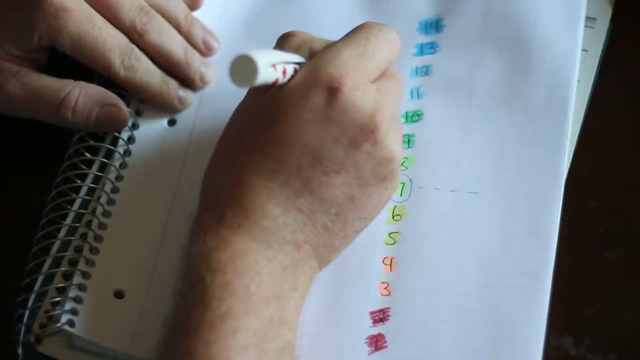 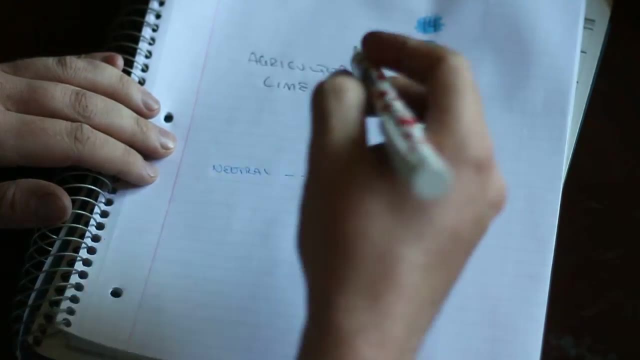 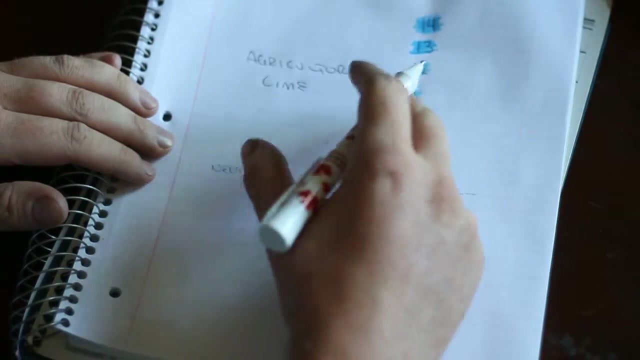 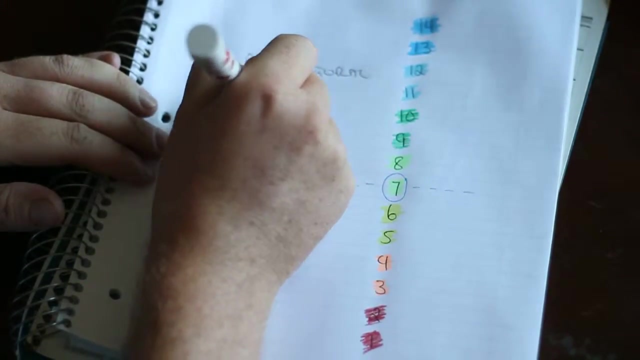 You can go with what is known as an agricultural lime And essentially what that is is just ground limestone And what that's going to do is it's going to slowly raise the alkalinity of your soil. It does this very slowly, but it's a much longer lasting process. If you wanted a quicker version of that, you can do hydrated lime. 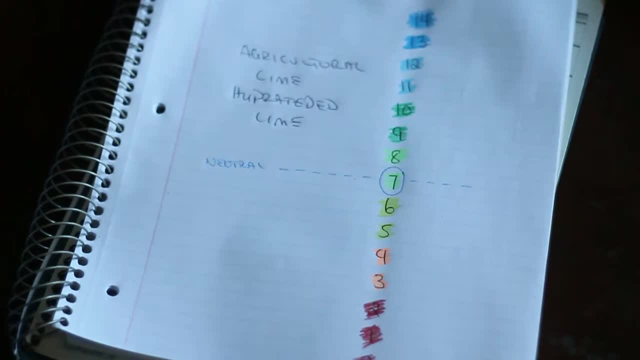 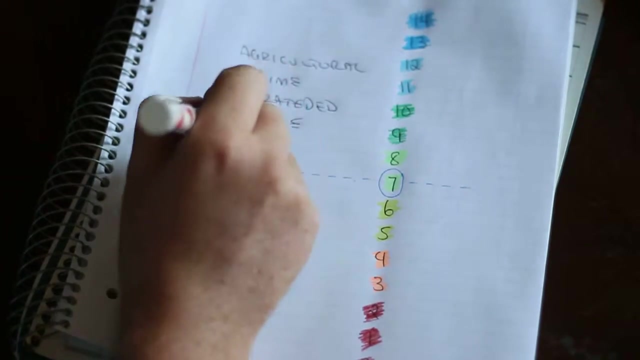 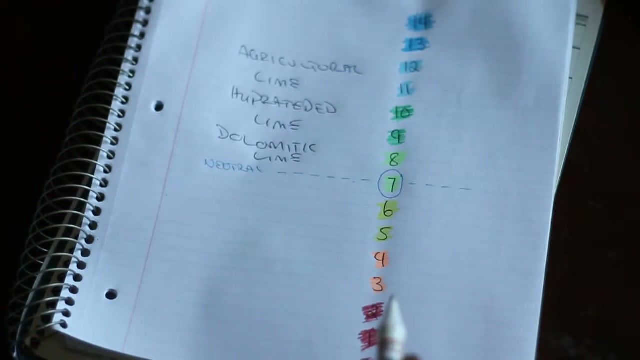 Hydrated lime is essentially what they do is they chemically alter the agricultural lime by adding water, And that is going to be a much faster acting but shorter lasting way to increase the alkalinity of your soil. You can also go with a dolomitic lime And what that does it's virtually the same as agricultural lime, but it's added magnesium, which plants do need. So if you find that it's going to be a good idea to go with that, 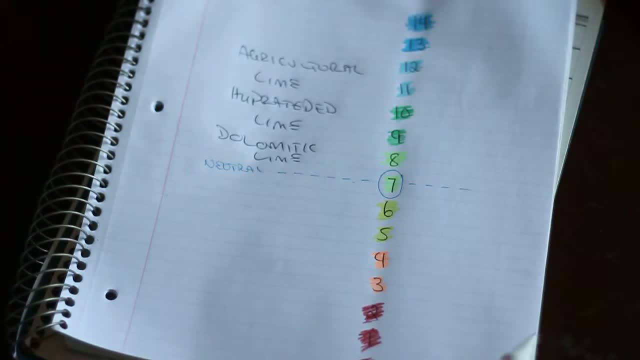 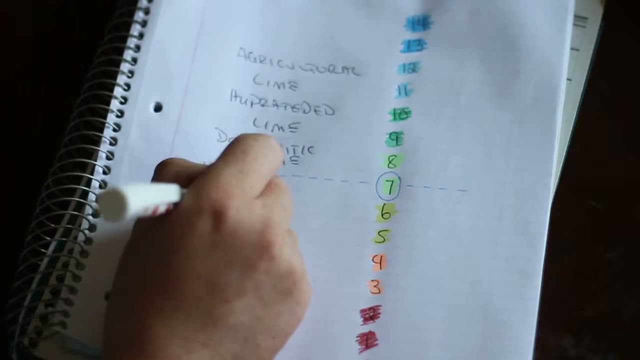 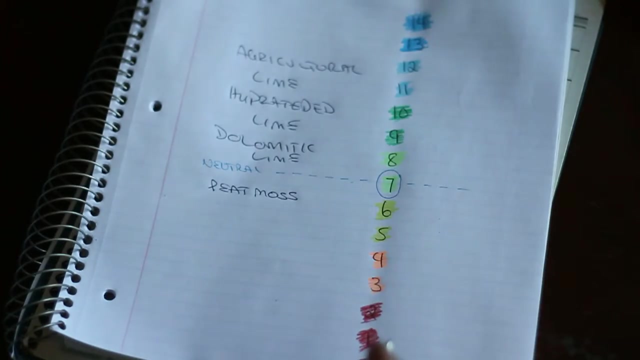 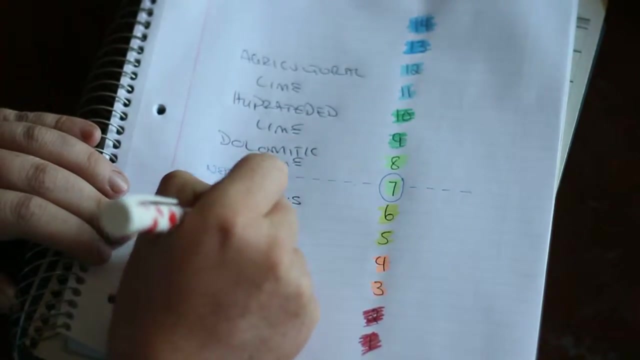 If you find that your soil is a little bit low on magnesium, you might want to opt for that. Now, when you're trying to lower the pH, my preferred method is going to be peat moss. I like peat moss because it's great for drainage. It also helps lower the acidity just a little bit. You can also use- excuse me, you can use- aluminum sulfate. 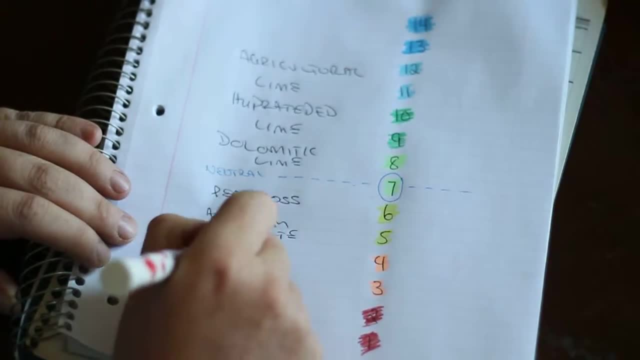 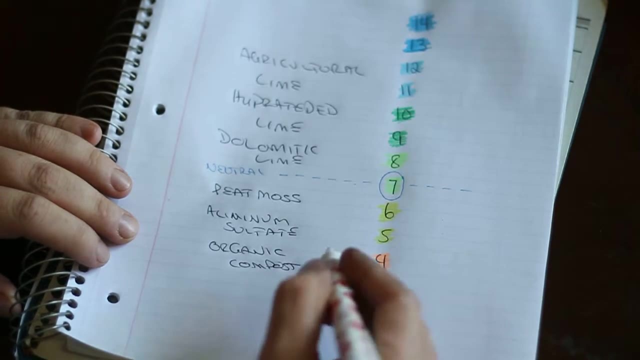 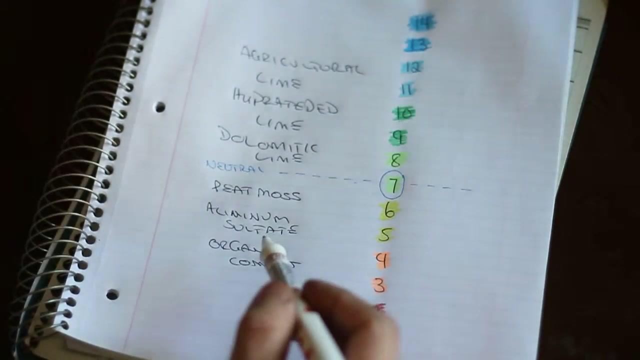 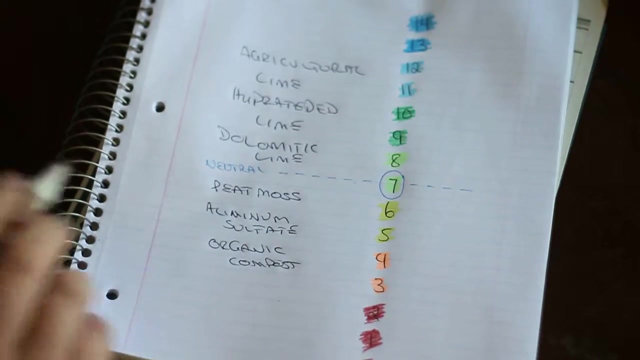 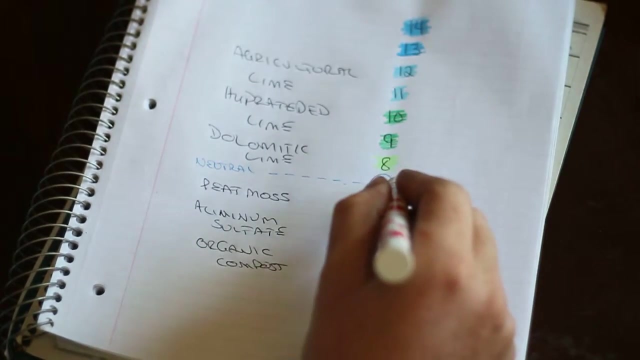 And you can also use just organic compost. Those three options, as well as a sulfur, are all going to help lower the pH balance, depending if that's what you want to do. Like I said, I prefer peat moss. The aluminum sulfate and the organic compost work just as well. It's just a matter of preference, Excuse me. So there are a few different plants that require a few different things. Most plants are going to be happy between about a six and a seven. 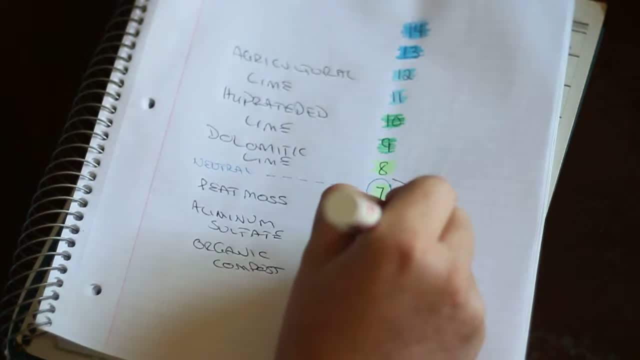 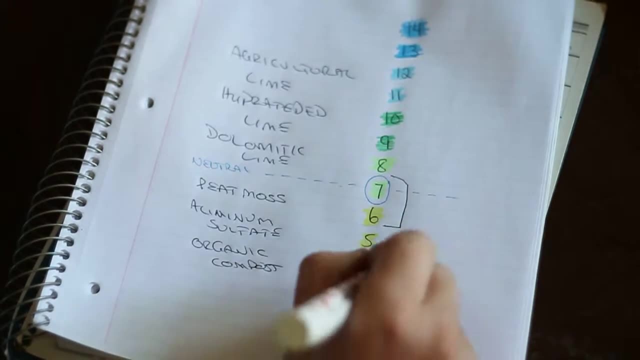 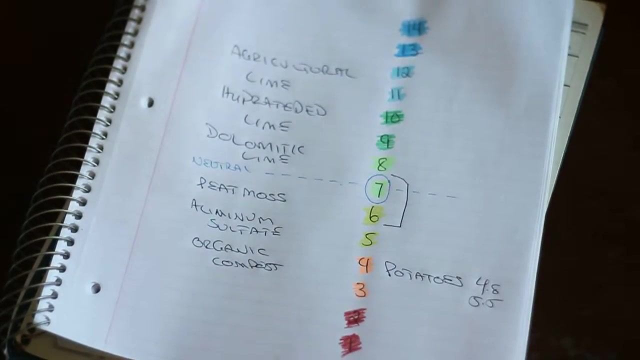 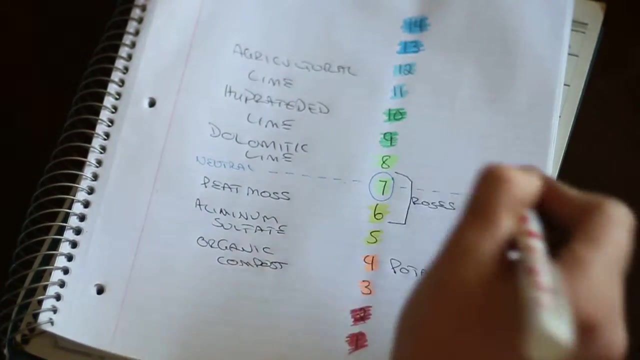 And a seven and a half rating. So somewhere in that range that'll be the majority of your plants. Just for example, you know potatoes are going to be about a 4.8 to a 5.5. So way more on the acidic side than most things. Roses are going to fall right in that sort of sweet zone. Rhododendron and azalea are going to be a good idea. 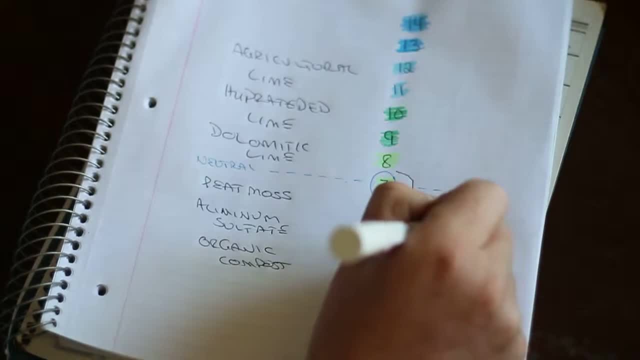 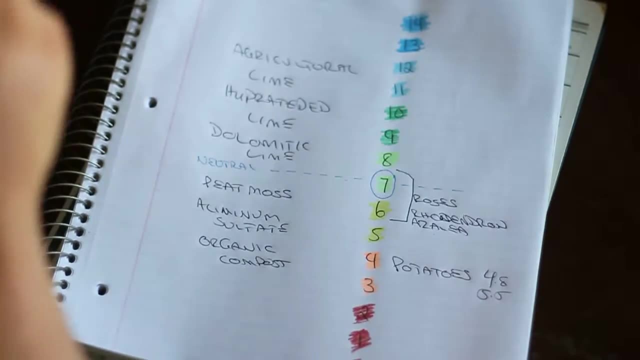 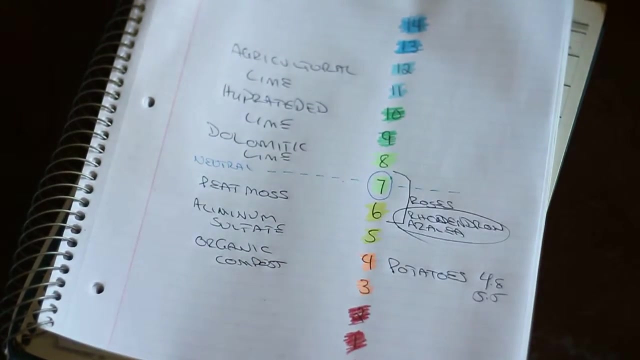 little bit less, but not too much, in around that 5.5 to 6 range. most of your fruits are gonna also fall sort of in this general 5.5 to 7 range, so your blueberries or raspberries, grapes, gooseberries, all that kind of stuff. 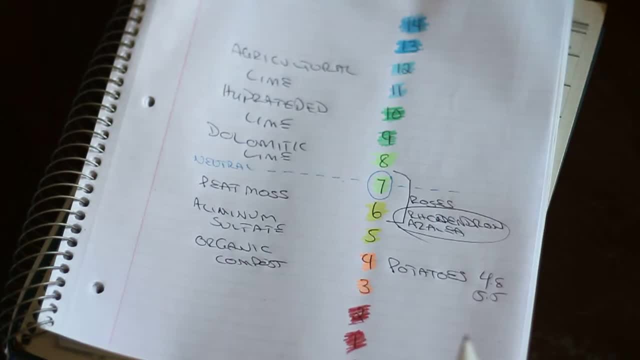 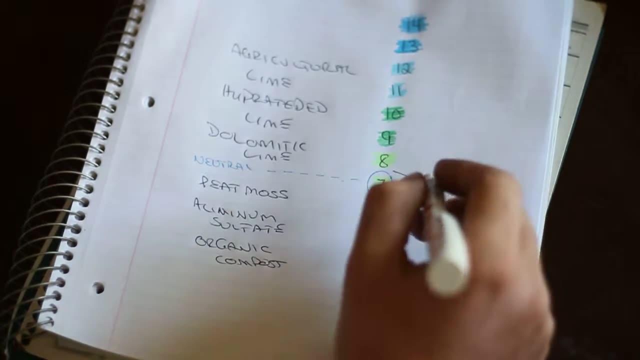 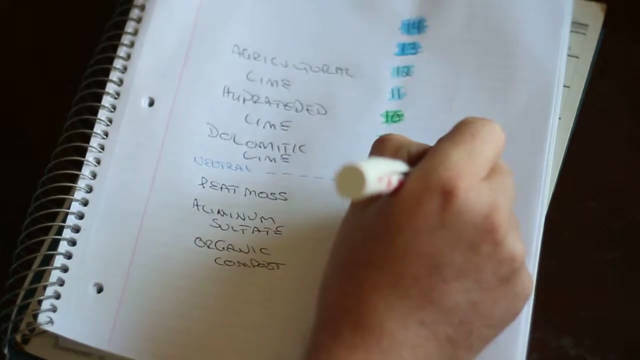 peppers, strawberries as well. those tend to be slightly towards that 5.5 to 6.5 range. if you wanted something slightly more neutral to alkaline, asparagus is going to be up around the 7 to 8 range. peaches plums- they also love a slightly. 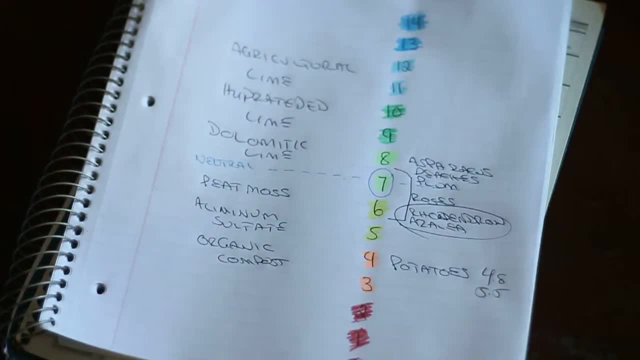 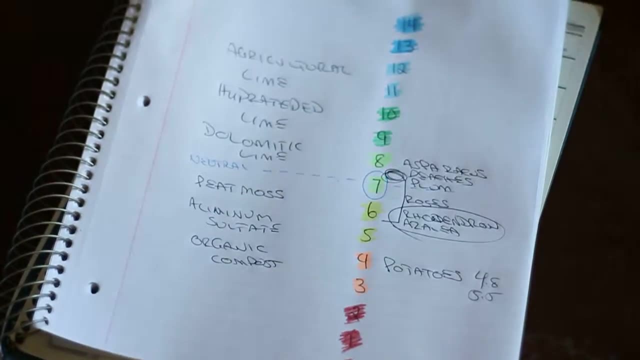 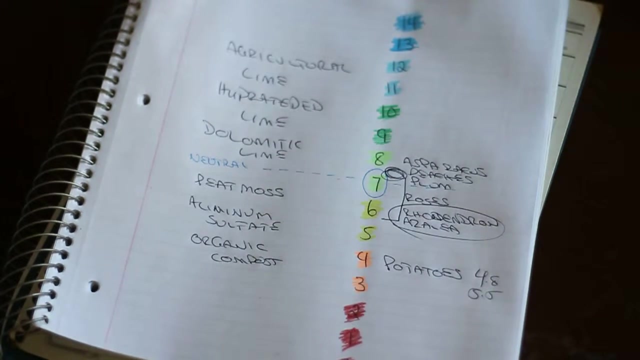 more neutral to alkaline. they're around that 6 to 7 range. brussels sprouts, beans, broccoli, they're all going to be sort of in this range here about the seven, seven and a half mark. so that's just a quick lesson on pH as well as a couple different ways how you can lower or 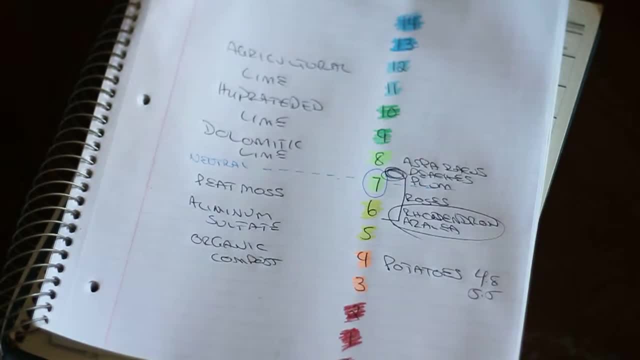 raise it depending on what you wanted to plant. I hope that was helpful and thank you for watching Garden Basics.